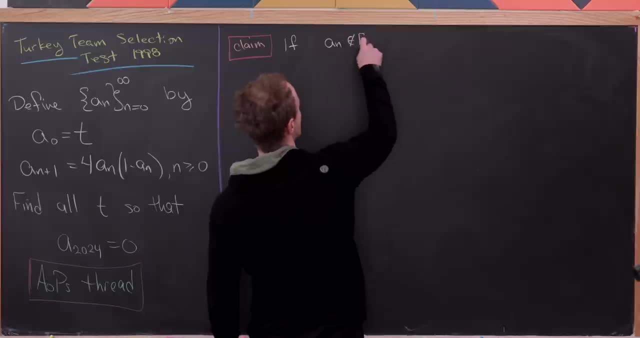 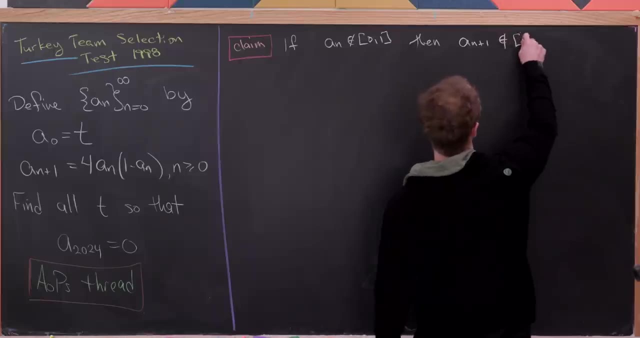 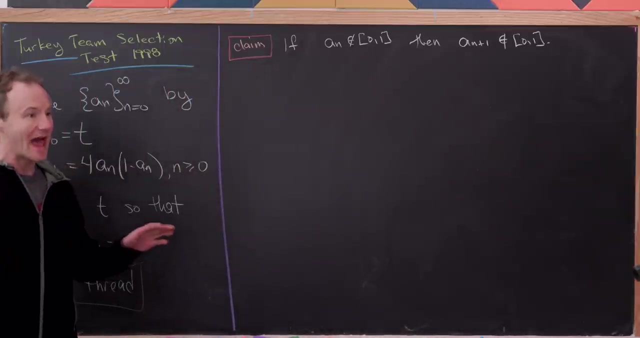 so if a n is not on the interval from 0 to 1, then a n plus 1 is Also not on the interval from 0 to 1. So well, that really tells us, if we ever get outside of the interval from 0 to 1, we never get back on that. 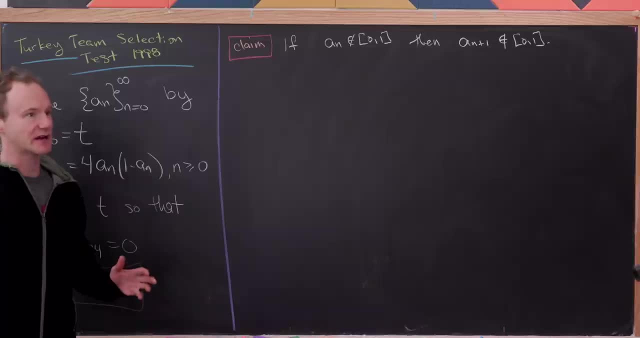 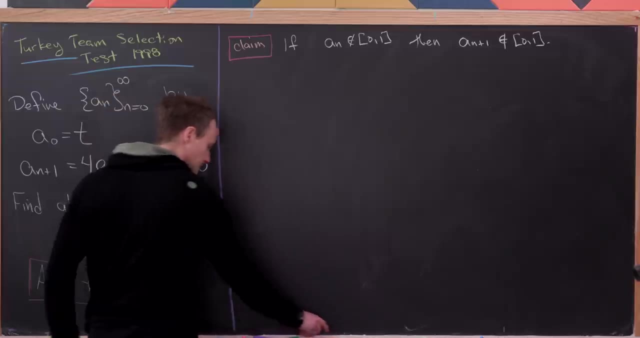 interval, And if we never get back on that interval, Then we can't ever be 0, because 0 is on the closed interval from 0 to 1. Okay, so let's see how the proof of this goes, and the proof is, you know, pretty straightforward. 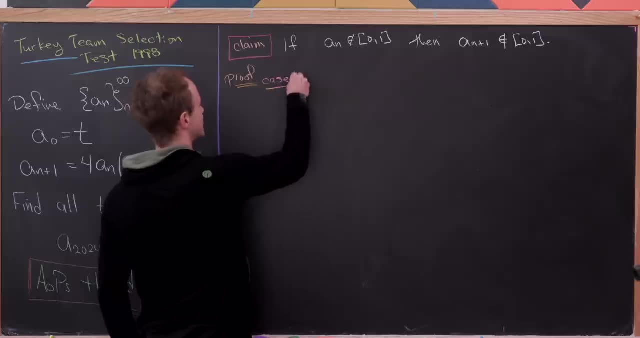 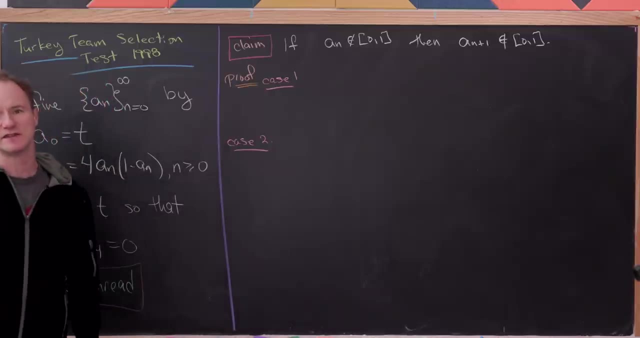 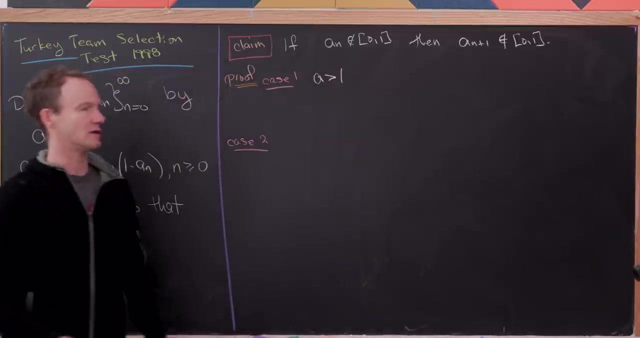 So we're gonna break this down into two cases and those cases, Well, are gonna be based off of which side of 0- 1 that you are on. So our first case will be: well, what happens if a is bigger than 0 or, sorry, bigger than 1, I should say. 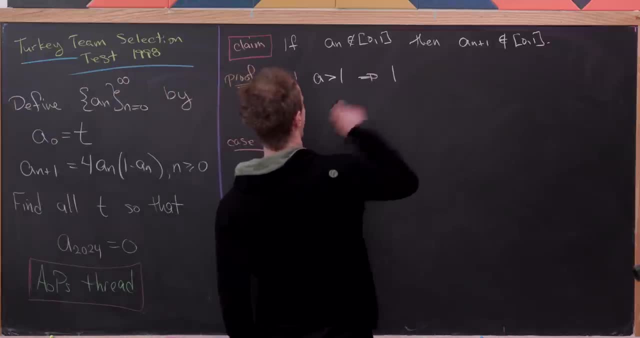 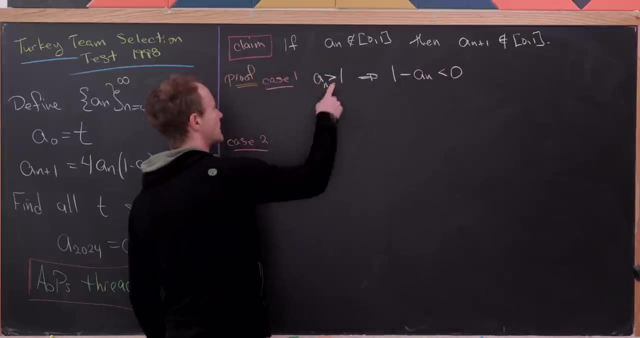 Well, if a is bigger than 1, then that means that 1 minus a- well, that should be a n. 1 minus a n is Less than 0, but, of course, if a n is bigger than 1, it's bigger than 0, and thus for a n is also bigger than 0. 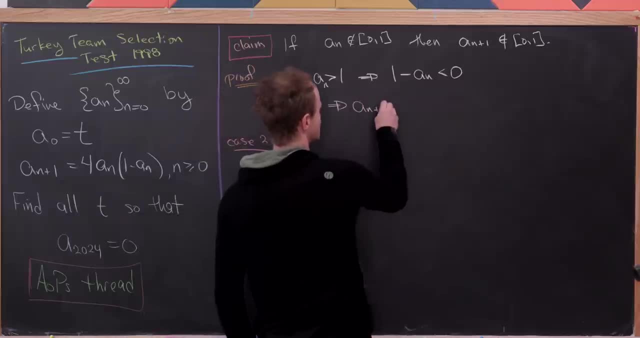 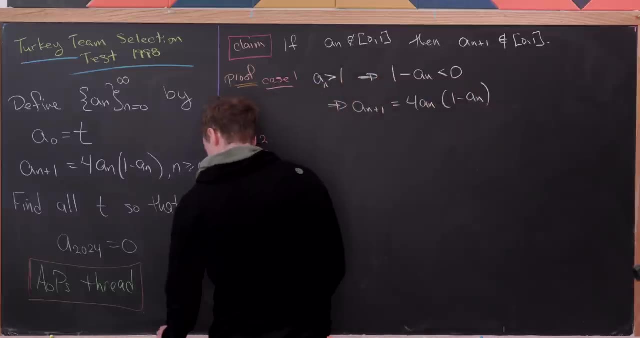 But then, putting these things together, we have a n plus 1. Well, that's equal to 4 a n times 1 minus a n. But now let's just look carefully at these parts. notice that this 4 a n is a Positive number by this assumption, and this 1 minus a n is a negative number. 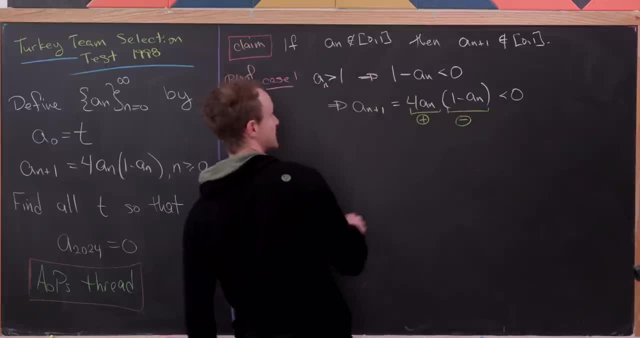 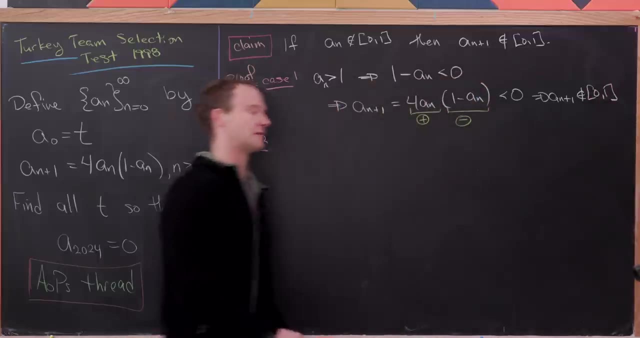 Making this whole thing a negative number, and thus it's less than 0. but if it's less than 0, then this a n plus 1 is outside of our interval from 0 To 1, so that's all there is to it in this case. 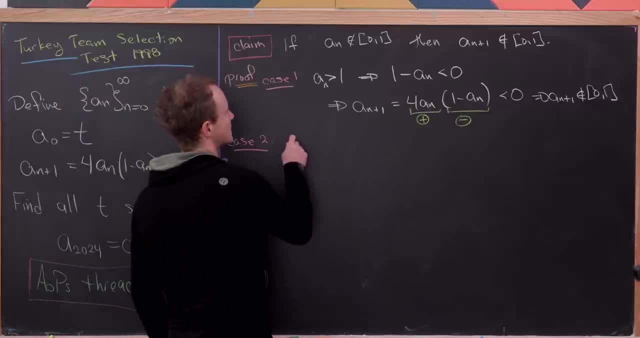 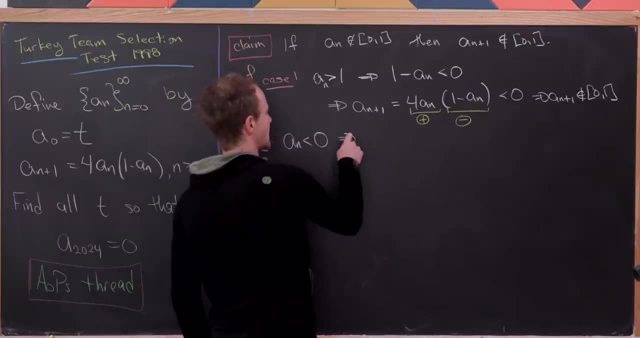 So now let's look at our second case, which is, of course, the case when a n is less than 0. That's the other side of 0- 1. okay, so if a n is less than 0, then 4, a n is also less than 0, and. 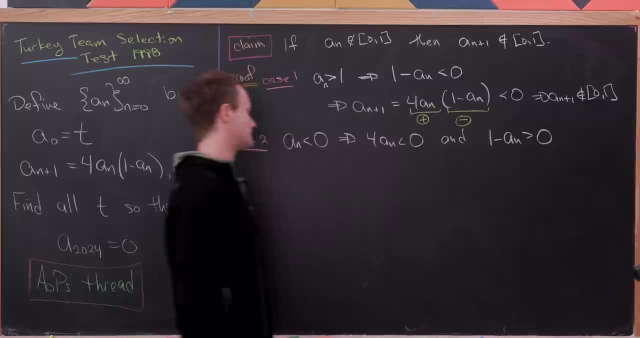 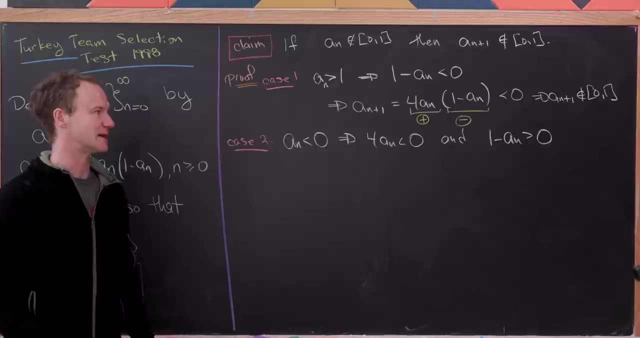 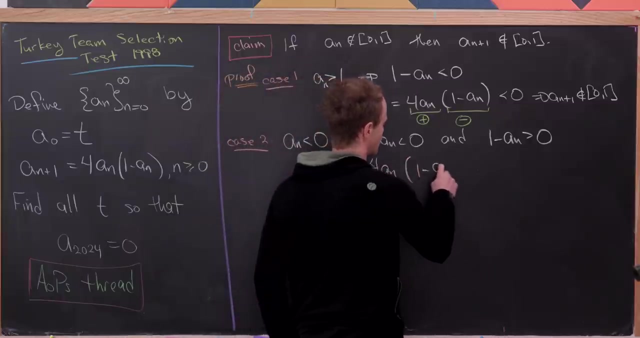 1 minus a n is bigger than 0. in fact, 1 minus a n is bigger than 1, But we don't really need that here, We just need that It's bigger than 0. But now let's observe that we have a n plus 1, which we can write as 4 a n times 1 minus a n. 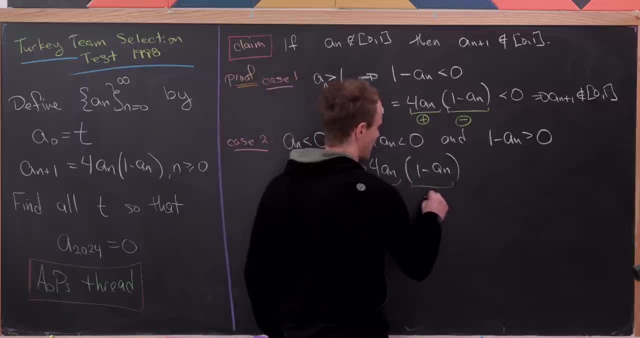 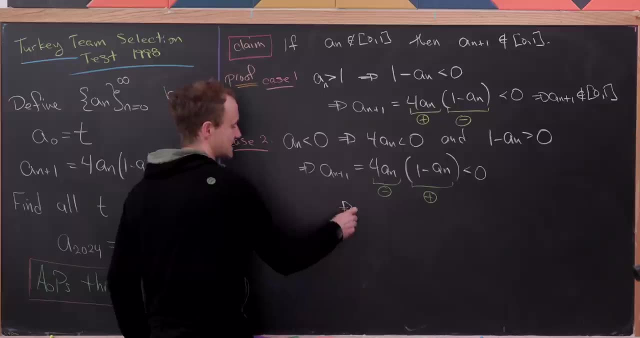 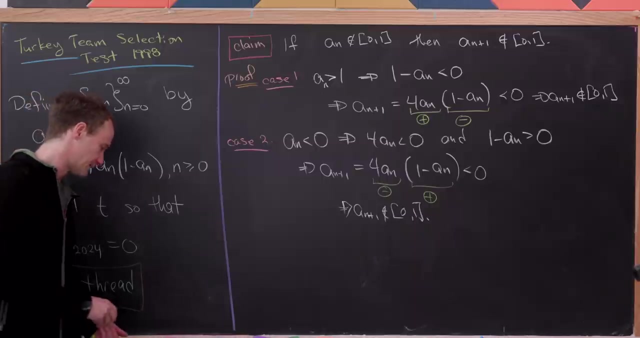 Now has a negative part first and a positive part second. but either way you look at it, It's less than 0. but if that's less than 0, then that means that a n plus 1 is outside of that interval. Okay, great, Now we don't exactly need this claim. 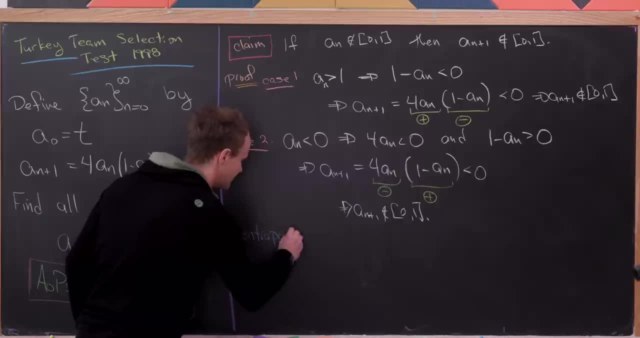 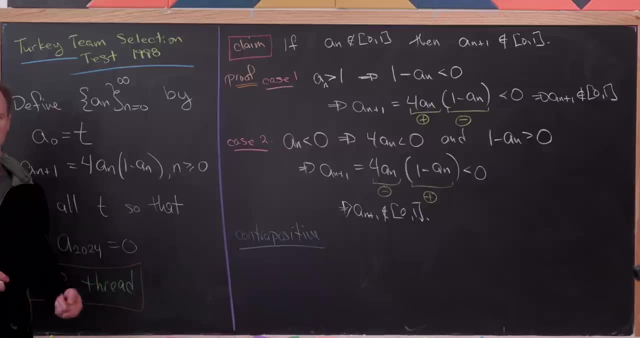 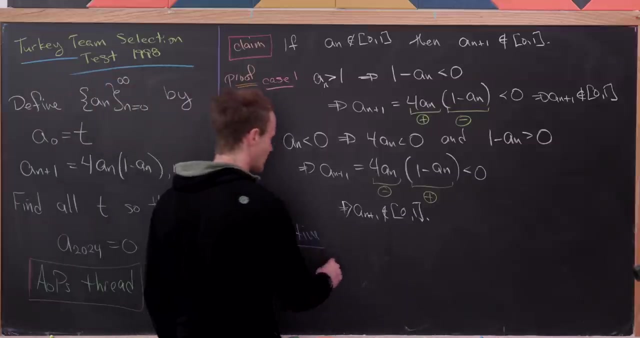 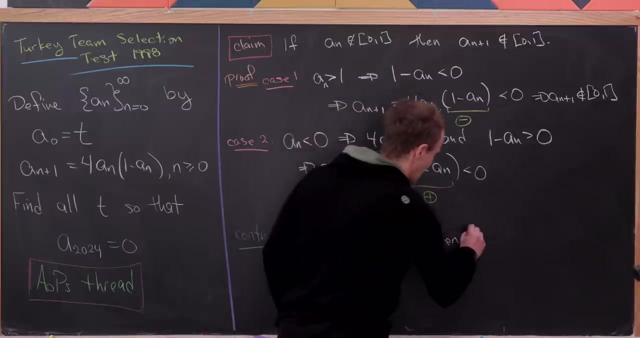 we actually need the contrapositive of this claim. So taking the contrapositive, well remember, contrapositive of P implies Q, is not, Q implies not P. So our contrapositive here would be: if a n plus 1 is on the interval from 0 to 1, then a n is on the 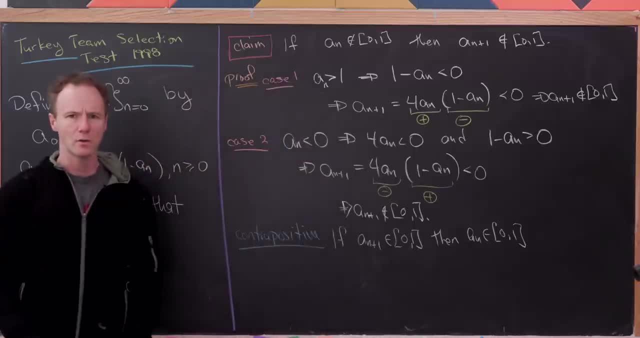 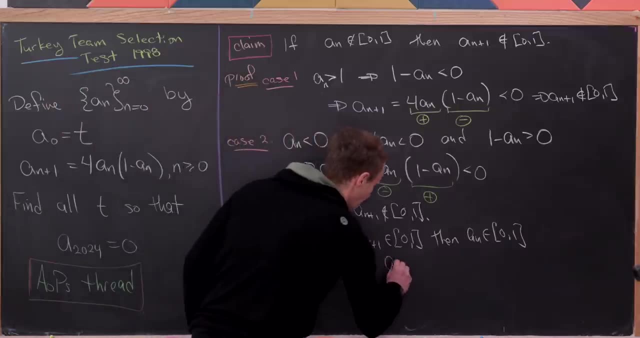 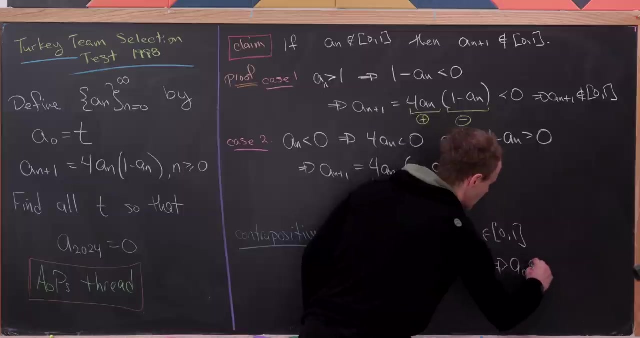 interval from 0 to 1.. But now we can just apply that over, and over and over again. So that is going to immediately imply that a n minus 1 is on the interval from 0 to 1, and on and on and on. a subzero is on the interval from 0 to 1.. 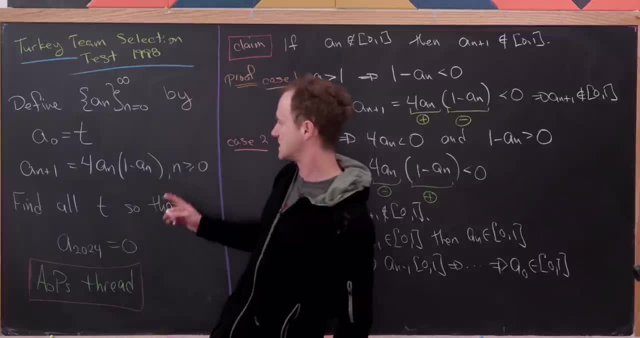 But in terms of our setupso if we want a sub 20- 24 to be misunderstood or nonsense, then we don't do the same thing. asalan地 and p胡 Slice again, But in terms of our setupso if we want a sub 20- 24 to be, 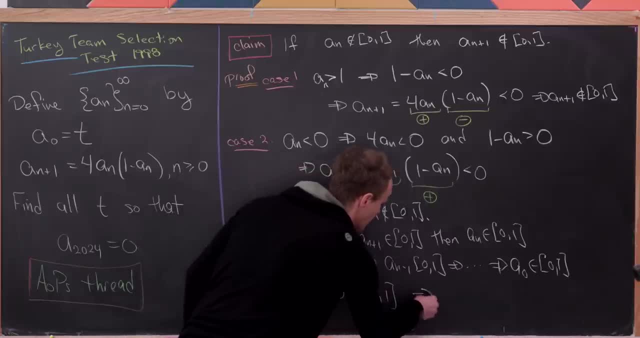 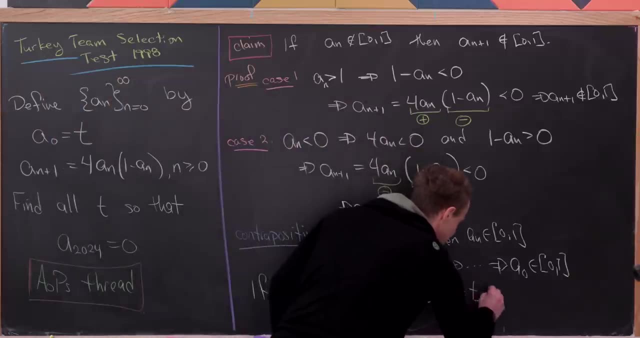 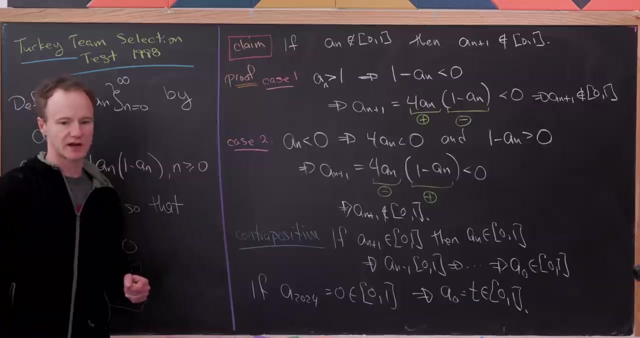 equal to zero, which is on the interval from zero to one, then that means all the way down at the ground we have a sub zero which is equal to t must be on the interval from zero to one. So that at least gives us a good starting place. so let's see where we can take that. So we just finished proving. 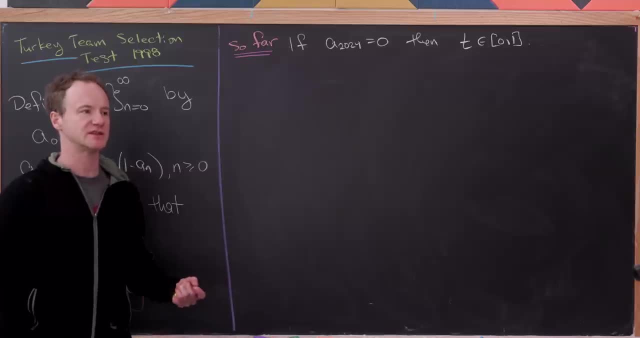 that if any element from our sequence is equal to zero, then the originating element of our sequence, the seed, if you will, had to be on the interval from zero to one. In particular, we're looking at the 2024th entry or element of our sequence, but, as you'll see, here we're actually really solving. 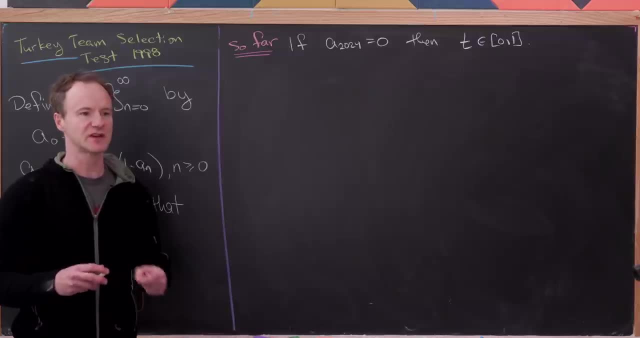 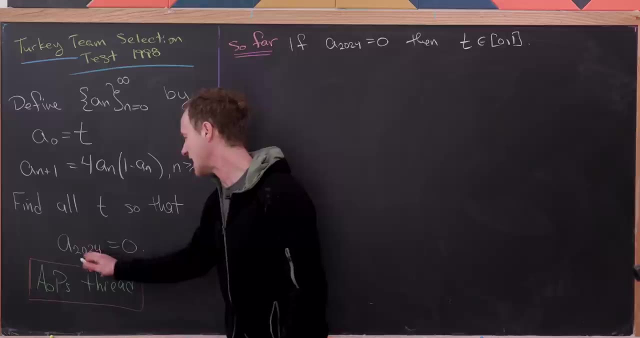 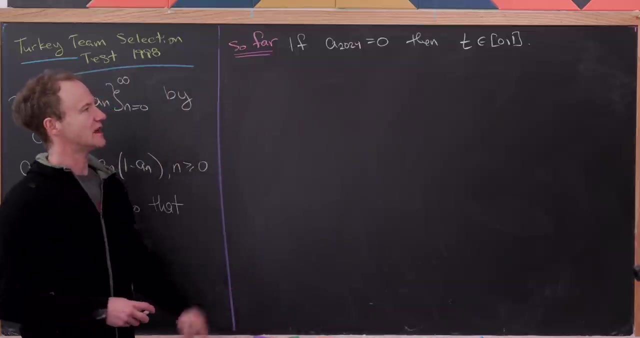 this in general. we're not writing it down in general, but this could easily be rewritten to answer the question: find all t such that a sub m is equal to zero for some fixed m? Okay, so anyway, let's get at it. So if t is on the interval from zero to one, then that means that there exists. 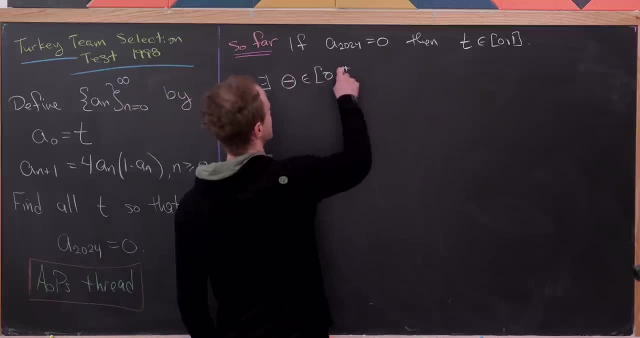 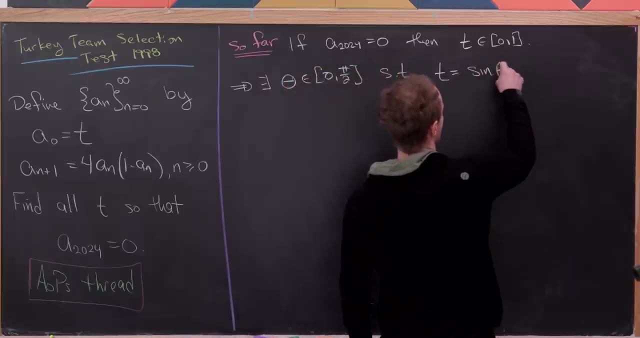 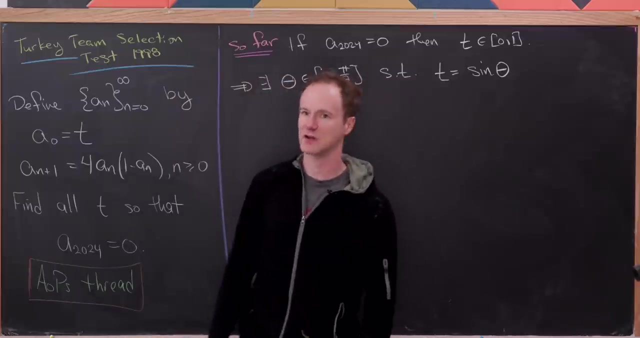 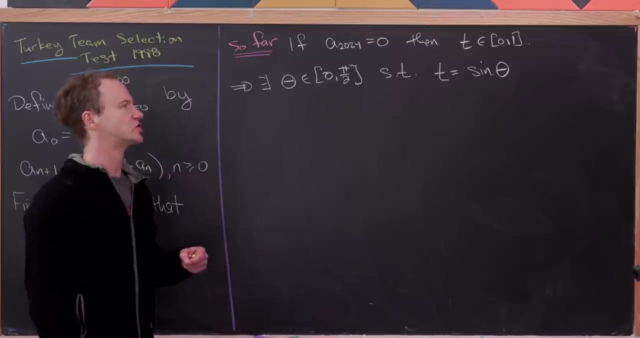 a theta on the interval from zero to pi over two, such that t is equal to the sine of theta. So this is where we're really leaning on this solution from this art of problem solving thread. I think this is a really nice approach. But now let's explore this a little bit and then we're going to tweak it. 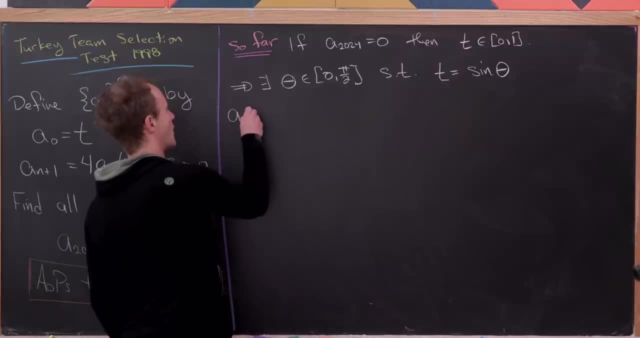 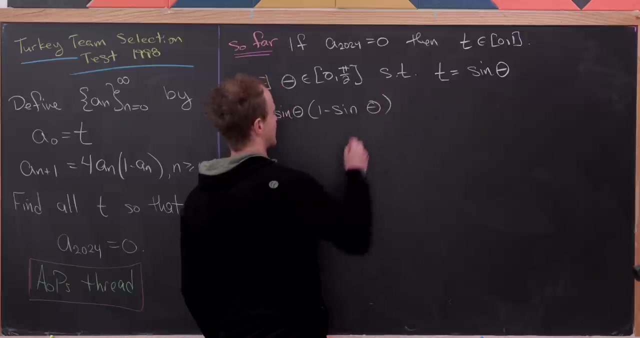 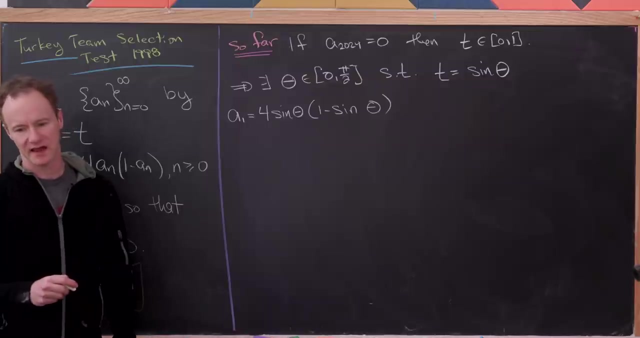 So notice, if t is equal to sine theta, then we have a. one is equal to: well, it's four times a zero, which is t times one minus a zero, which again is t. So we have four times sine theta times one minus sine theta. Okay, well, how could this simplify? Well, I look at that one minus sine theta and I think: 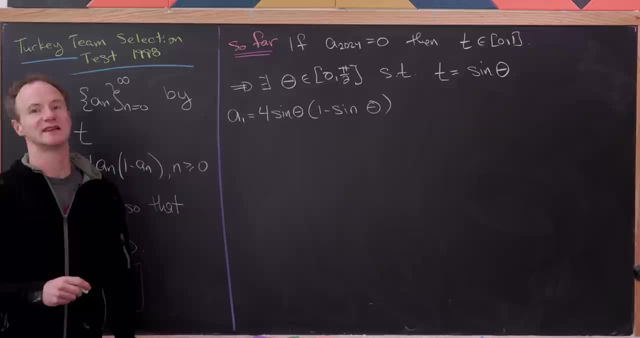 well, I really wish that was one minus sine squared theta. then I could turn it into cosine squared theta using the Pythagorean trig identity. But in fact we can do that because since sine theta is one to one and on two, from zero to pi, over two up to zero to one, sine squared is also one to one and 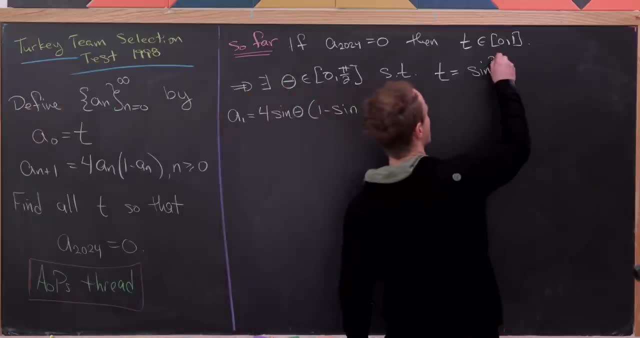 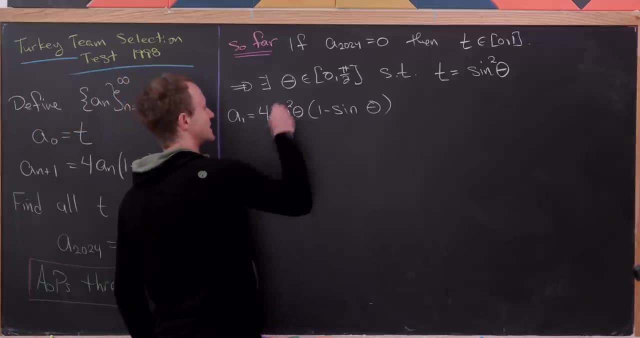 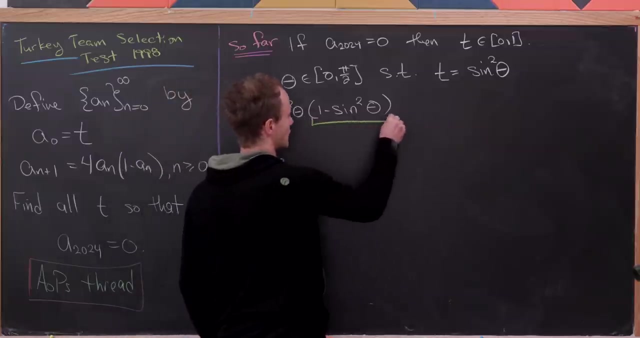 on two on that interval. So we might as well parametrize this as well. So let's look at this number t by sine squared theta instead of sine theta. So that's going to turn this into four times sine squared, times one minus sine squared. and well, I'm just going to write real quick that. 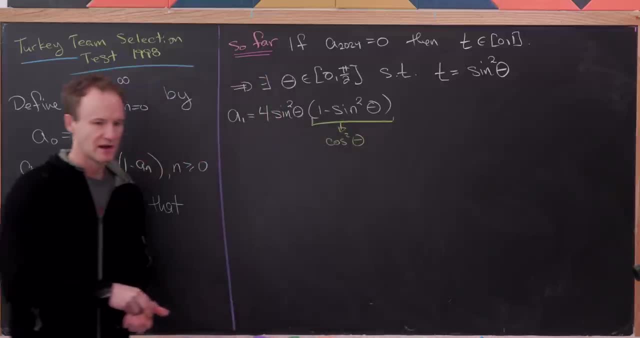 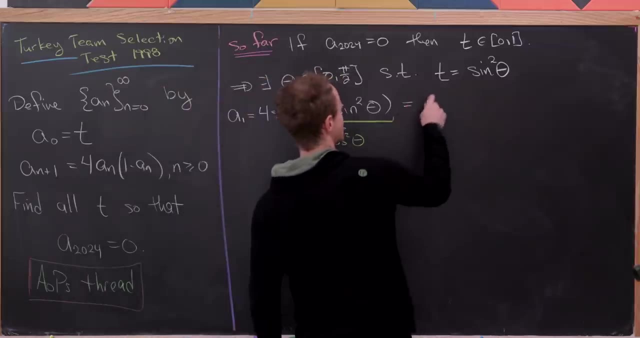 this is equal to cos squared theta, But of course that's why we introduced the sine squared in there in the first place. But now we can factor the square out of the whole thing and we have two times sine theta, times sine squared theta. So that's going to turn this into four times sine squared. 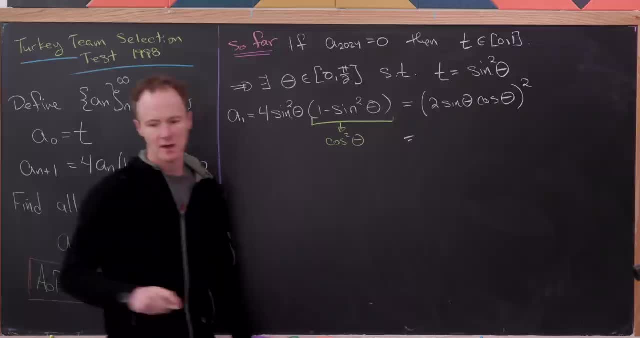 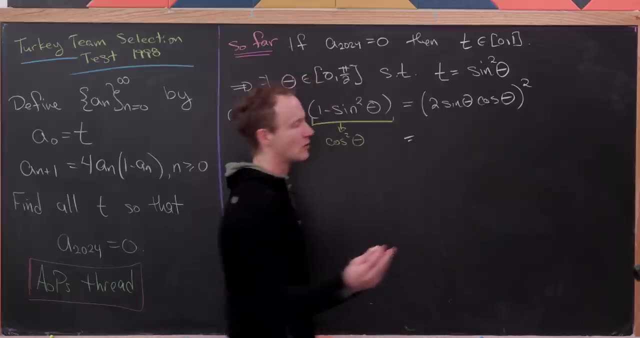 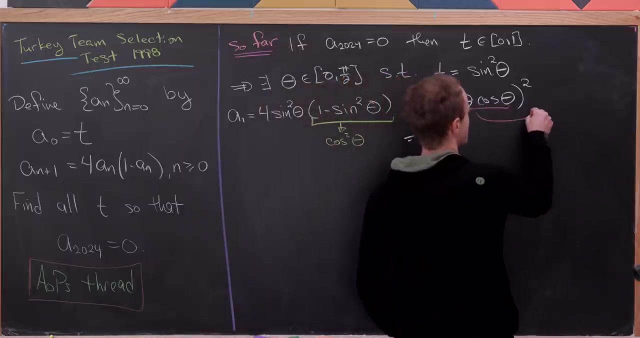 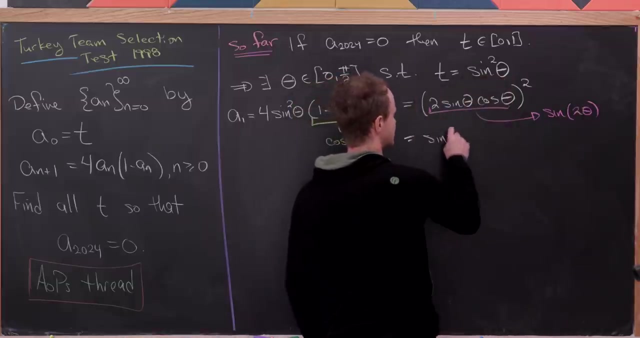 times cosine theta, quantity squared. But now that's in fact a trigonometric identity and the trig identity that is, is a double angle formula for sine. So in fact this stuff that's being squared is equal to sine of two times theta. So here we have: this is equal to sine of two times theta. 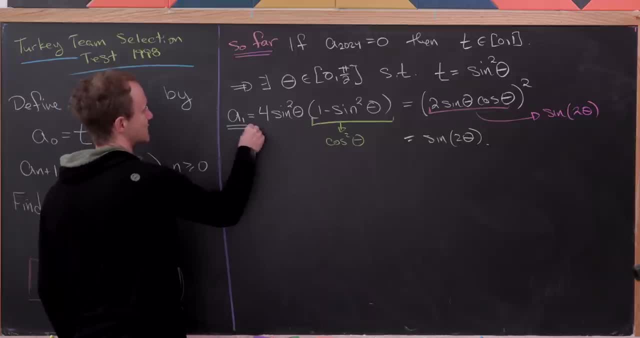 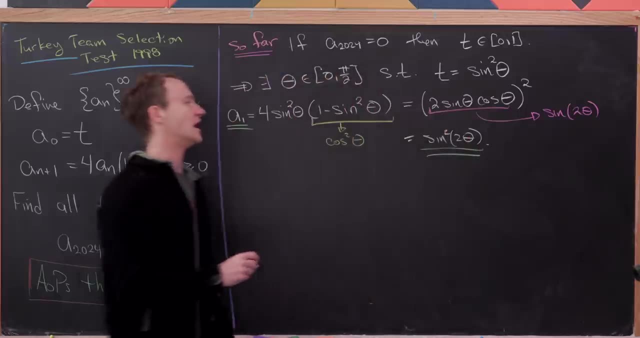 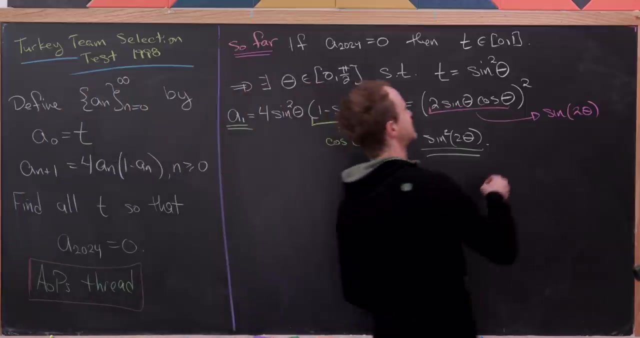 Okay, so let's see what we get. We have a sub. one is equal to sine squared, I should say, because that was inside of the square of two times theta. Now let's see if we can generalize this a little bit. and in fact it's. 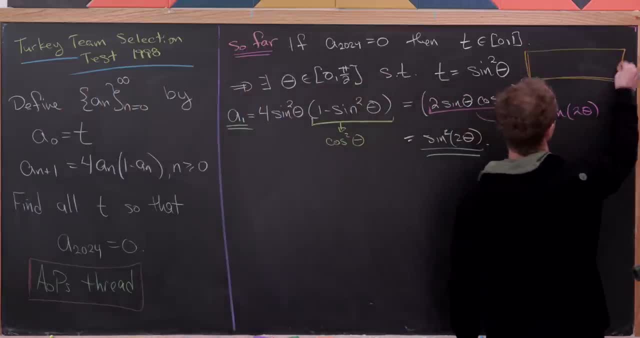 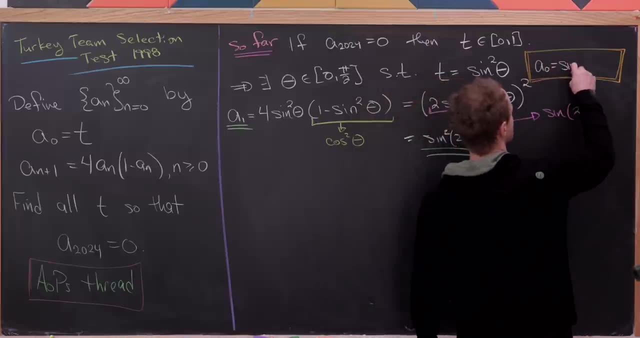 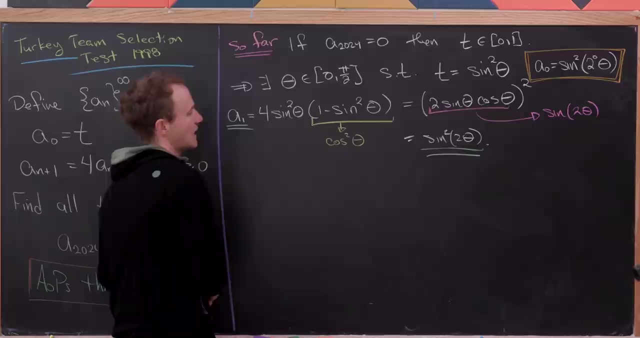 not that big of a leap if we go back up here and rewrite this t equals sine squared theta as a not equals sine squared of two to the z Zero times theta, And then we go ahead and rewrite this thing that we've derived with a. 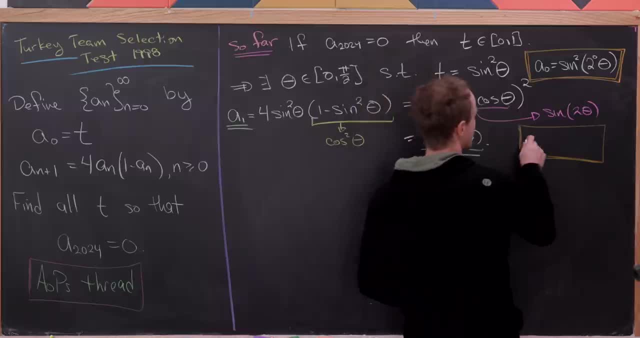 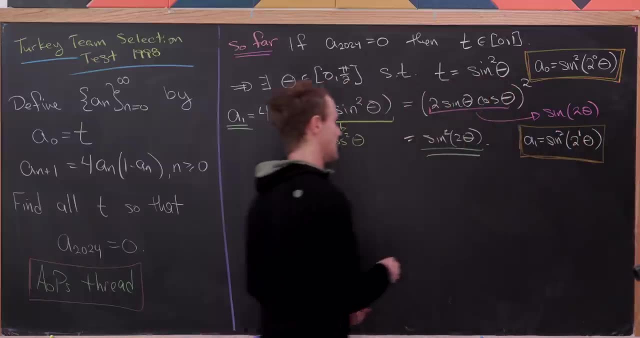 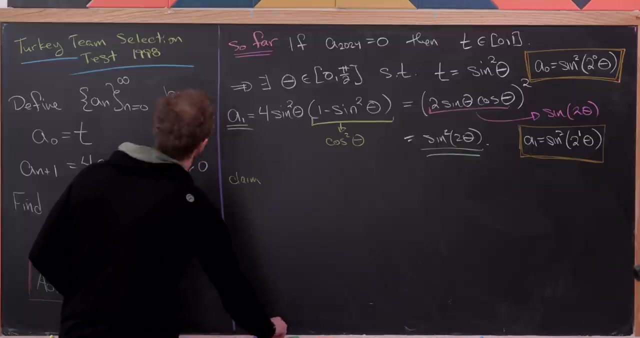 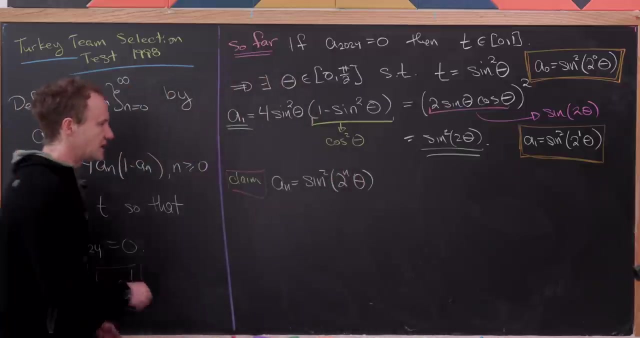 one, as, let's see, a sub one equals sine squared of two to the one times theta, And that really brings us to you know, what I'll call an obvious claim. And that obvious claim has to do with, well, the first area of the solar system. So the first area of the solar system is the 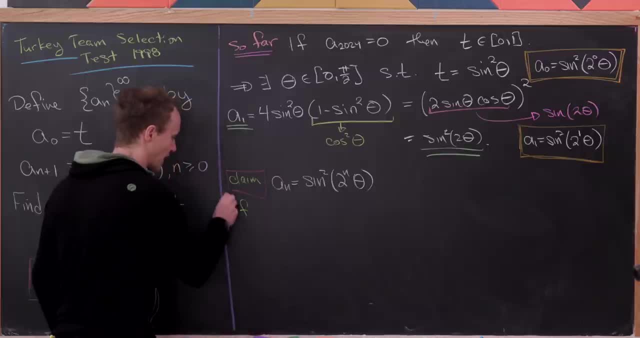 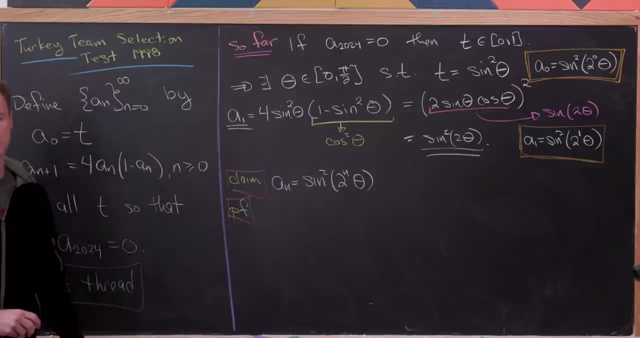 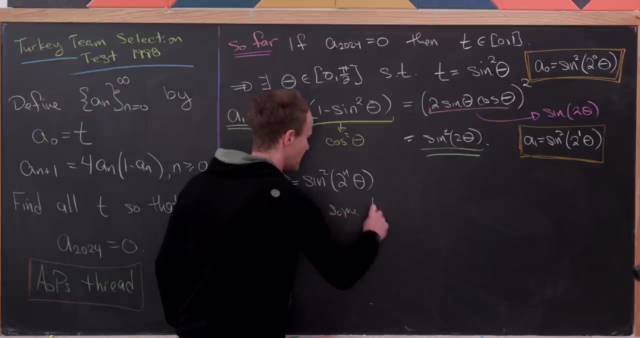 integral of sine squared of two to the n times theta. So you have the integral of sine squared of two to the n times theta. Now of course, you know, if we want to prove this, which we will prove this- we probably want to use induction, The base cases totally taken care of by either of those. now we just need to do the induction step. so let's suppose for some K bigger than or equal to, 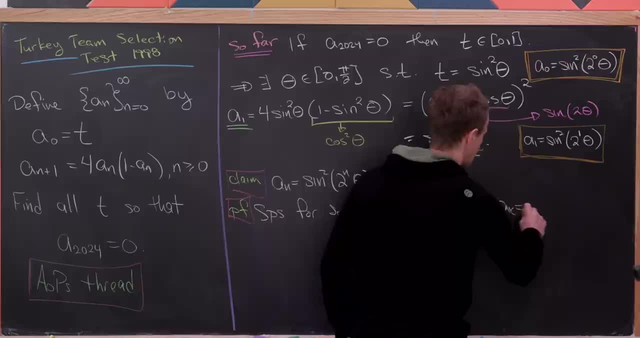 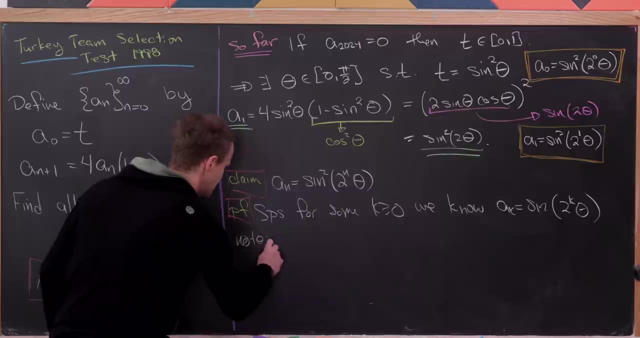 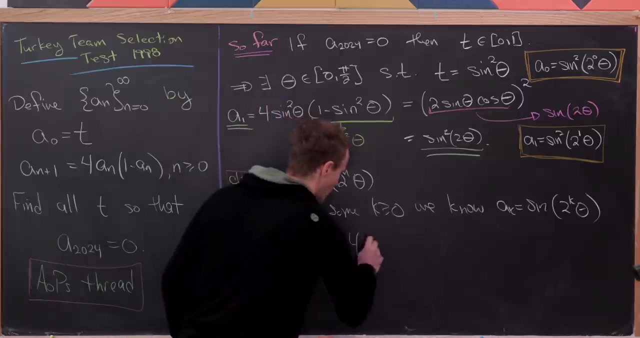 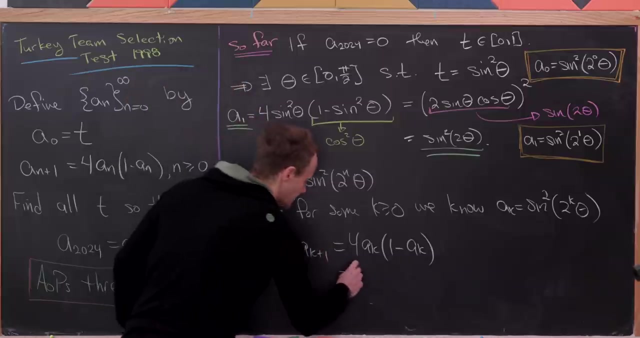 equal to zero, zero. we know a sub k is equal to sine of two to the k times theta. and then, well, let's just do the calculation we have: a sub k plus one is equal to four a k times one minus a k. oh, and i keep forgetting my squared here. so that's going to be four sine squared two to the k times. 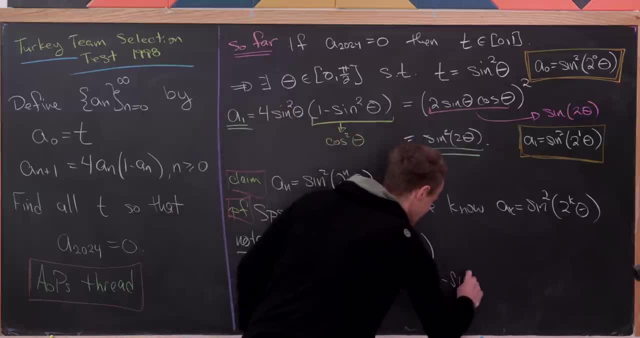 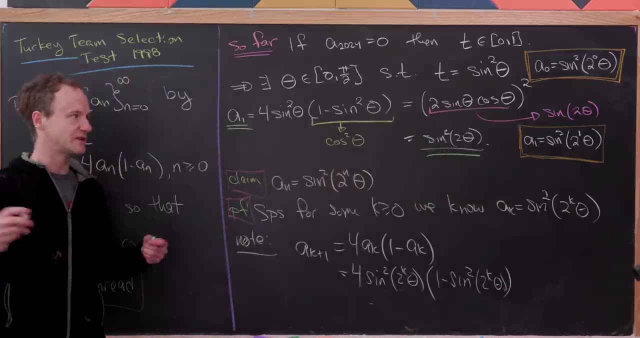 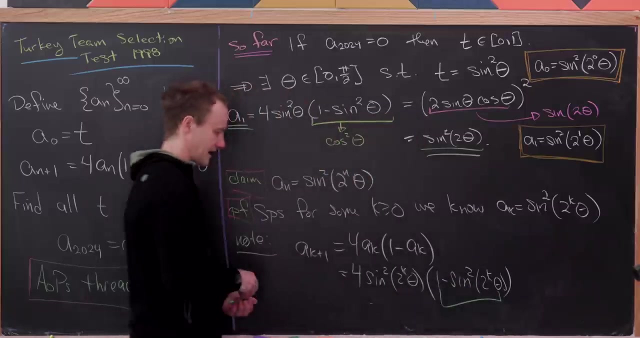 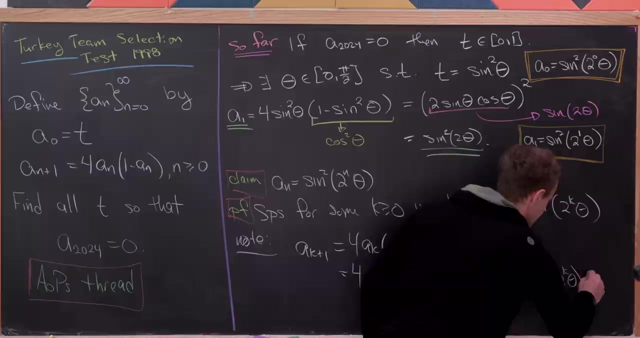 theta and then one minus sine, squared two to the k times theta. but then factoring the square out of the whole thing, then using the pythagorean trig identity on this thing- and i'm underlining in green- will give us two times sine, two k theta times cos, two k times theta all squared. 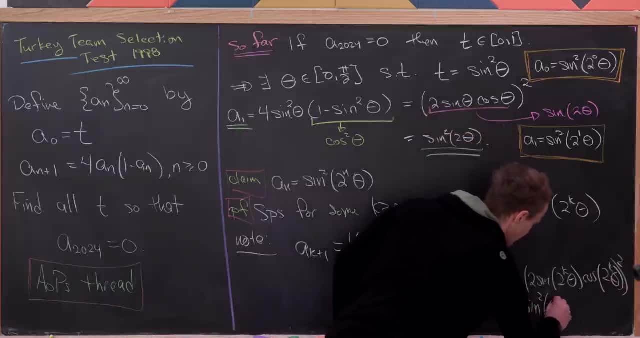 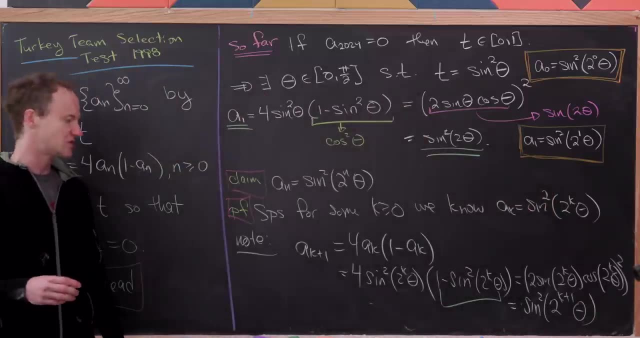 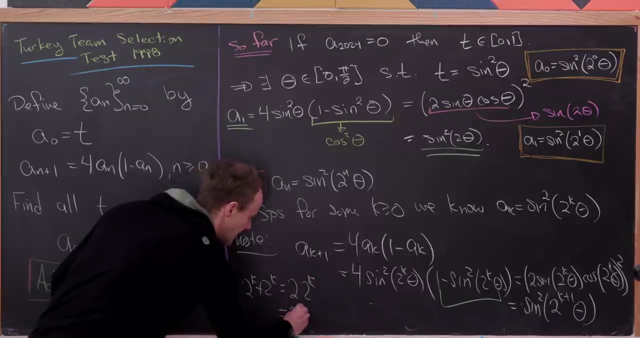 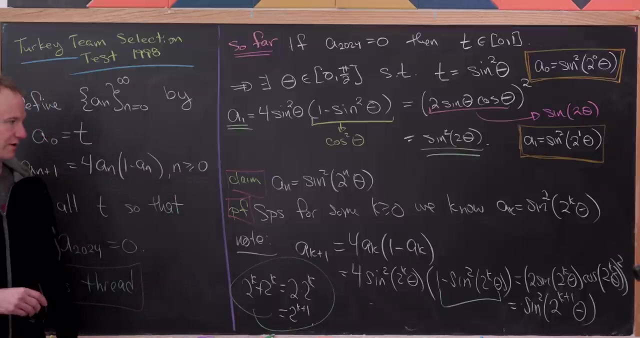 but of course that's going to turn into sine squared of two to the k plus one times theta, using double angle formula, and the fact that two to the k plus two to the k is two times two to the k, which is two to the k plus one. so we use that little like simple arithmetic, you know, in inside of that problem over. 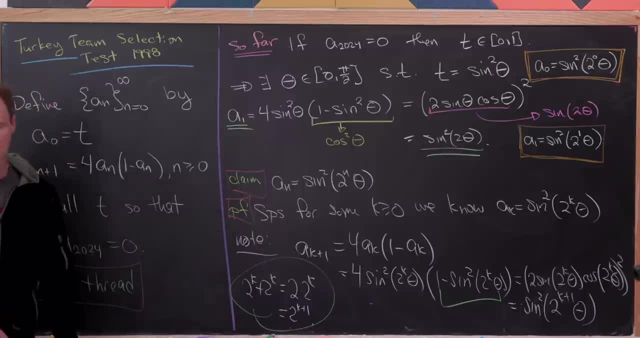 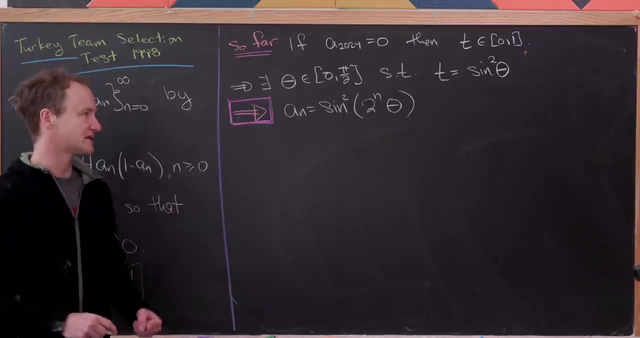 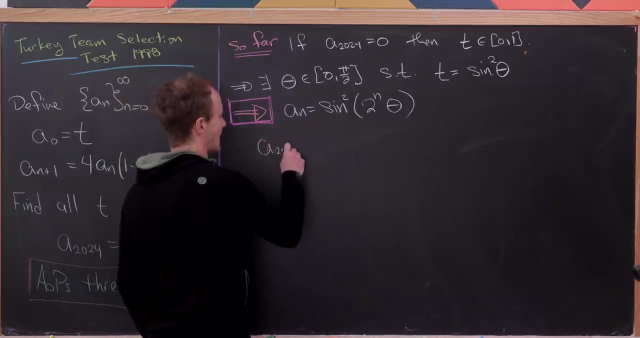 there. okay, great. so now we've got this closed form for a, so then let's see how that finishes it off, basically. so we just proved that our sequence has this nice closed form as sine squared of two to the n times theta, that's the nth term. okay, so let's note that we want a 2024 to be equal to zero, but 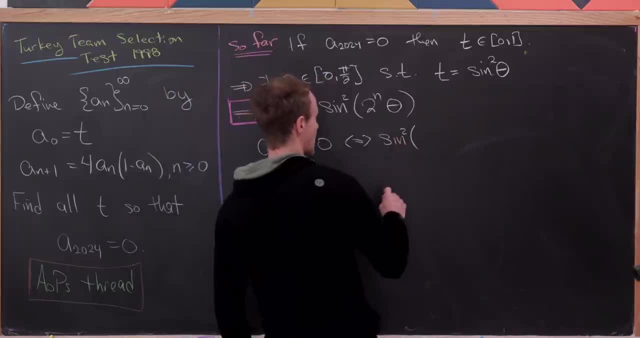 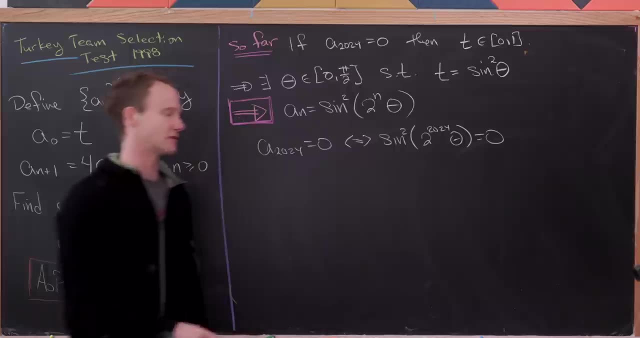 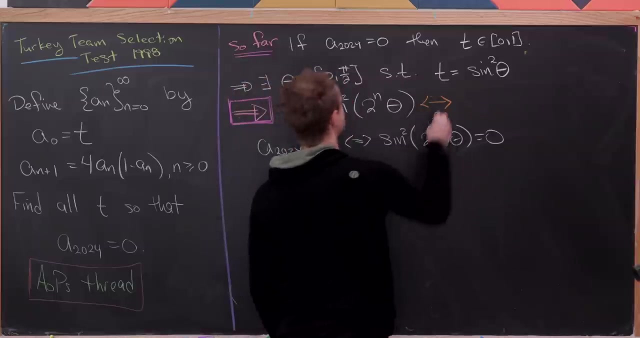 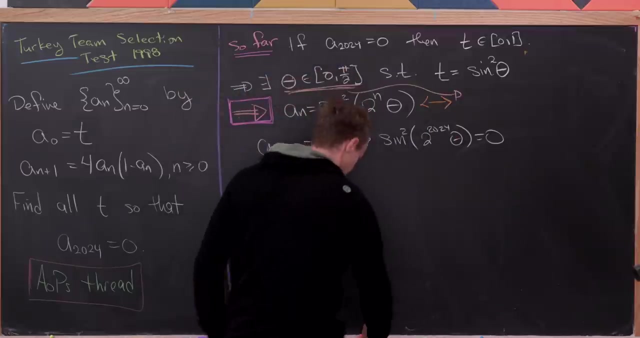 that's of course equal to zero if, and only if, sine squared of two to the 2024 times theta is equal to zero. but now let's go up here, one line above, and observe that since theta is between zero and two pi, that means that two to the n times theta. 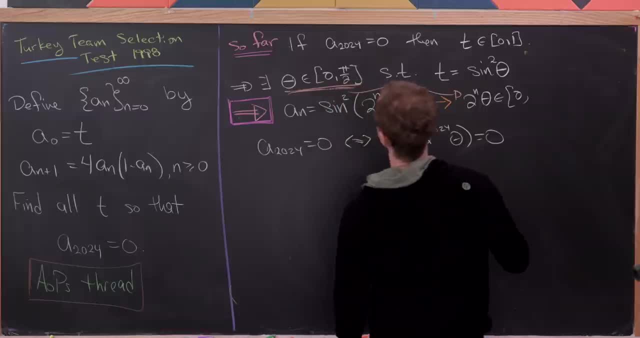 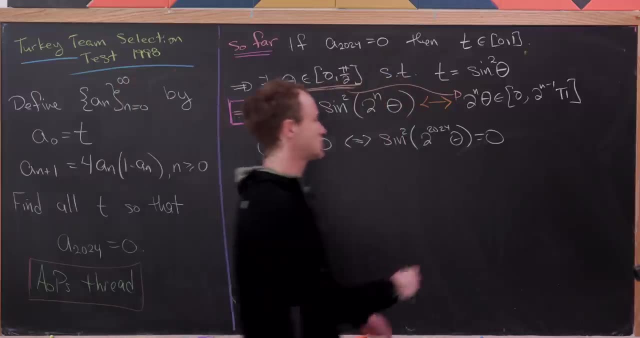 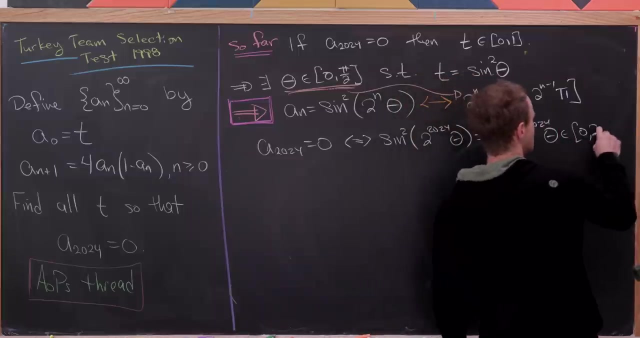 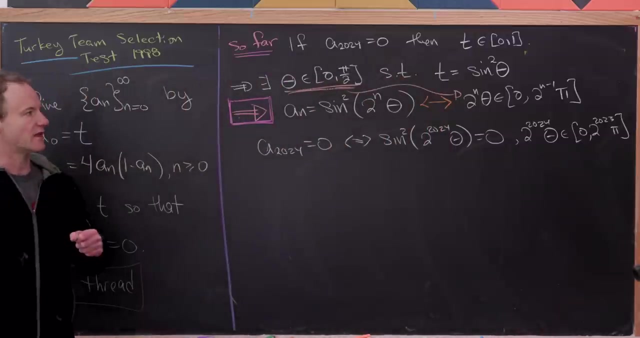 is between zero and let's see two to the n minus one times pi. so specialized down here we have two to the 2024 times theta is on the interval from zero to the n minus one times pi. so that's zero to two to the 2023 times pi. but of course we know that sine is equal to zero, exactly on the. 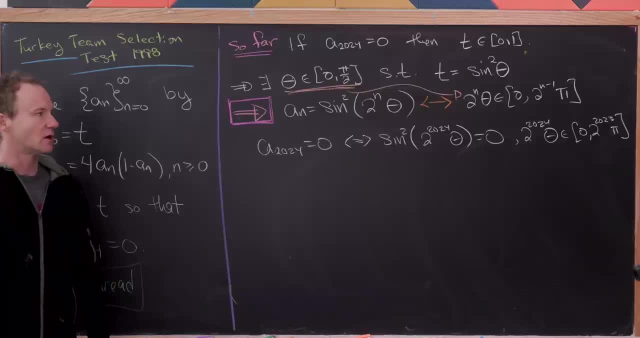 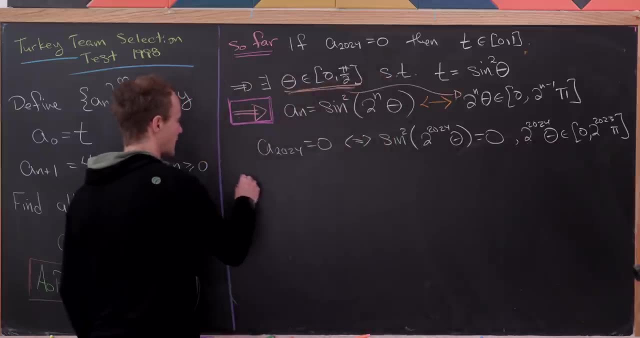 integer multiples of pi. so what we need to do is look at the integer multiples of pi on this interval, and that'll be exactly where this sine squared of that stuff is equal to zero, so that means two to the n times theta is equal to zero, so that's two to the n minus one times pi, so that's. 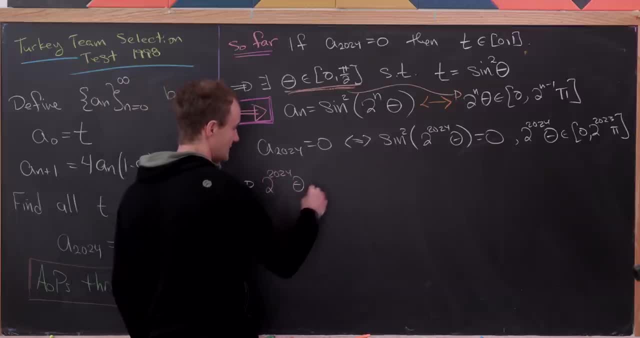 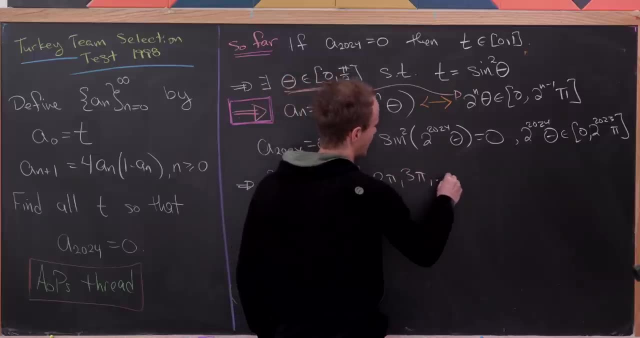 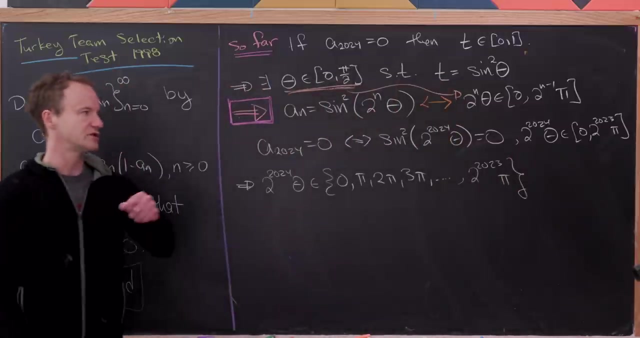 great. so we know that sine squared of two to the n is equal to n minus one, so that's zero, and that's plus one pi, so that's four pi, and five, that's three pi. so that's class화 square. we've overả ratio here of sine to the n times pi and hisПрx and residence Agora. 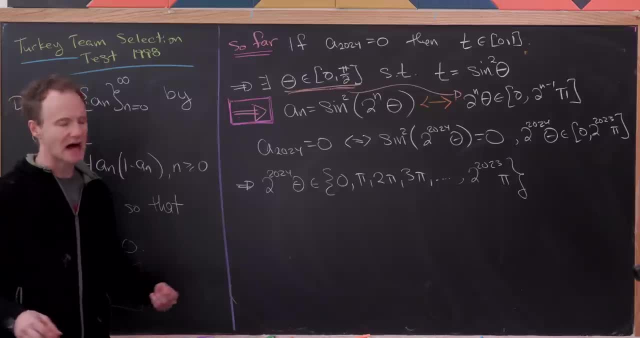 wire to know that sine squared of two to the n minus one is equal to zero. so we take hooray color, so that does work, for the n minus one being equal to zero. basically, what we want to do here is we want to cancel out. So now, well, we can just divide everything by 2 to the 2024, and we have the values of. 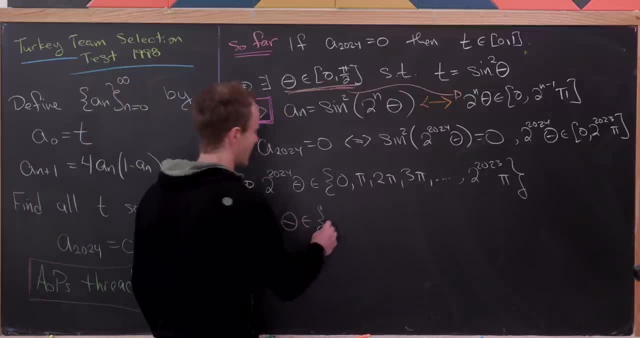 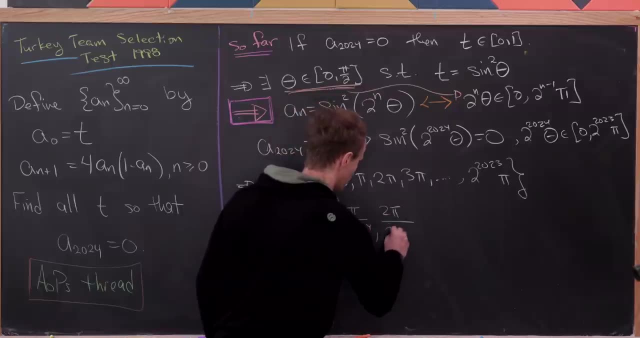 theta. So that means theta is from the set 0 pi over 2 to the 2024,, 2 pi over 2 to the 2024,, 3 pi over 2 to the 2024,, 4 pi over that, 5 pi over that, so on and so forth all the way. 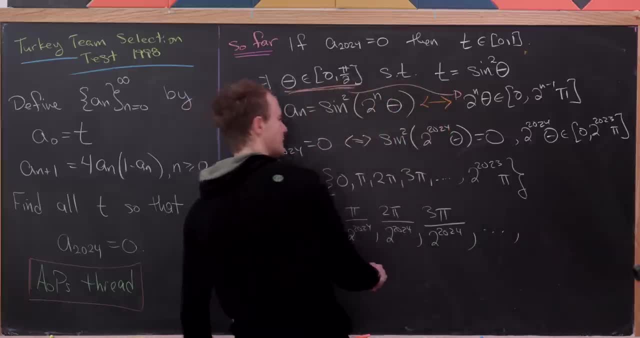 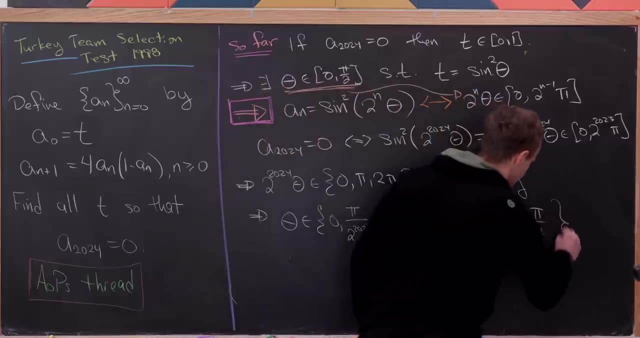 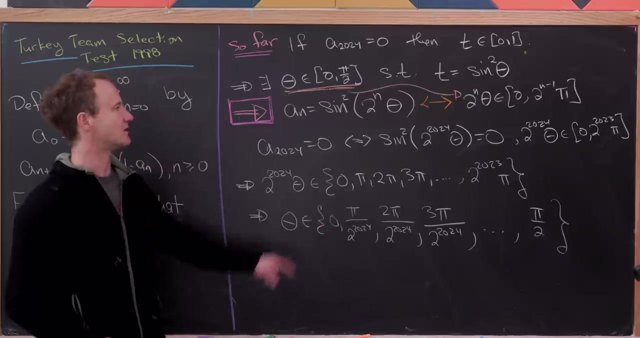 up to 2, to the 2023 pi over that, which is going to give us pi over 2.. Great, So notice, we've got this kind of nice equal distribution of values of theta between 0 and pi over 2, which were the values that were allowed anyway. 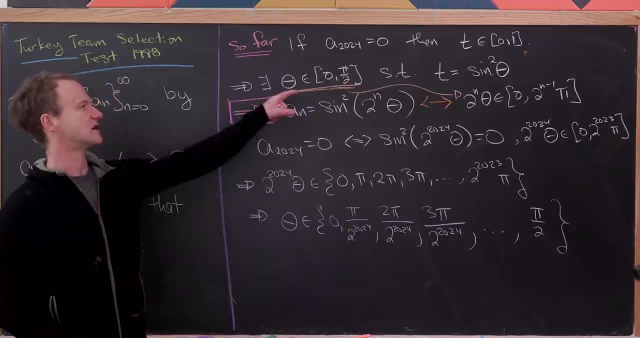 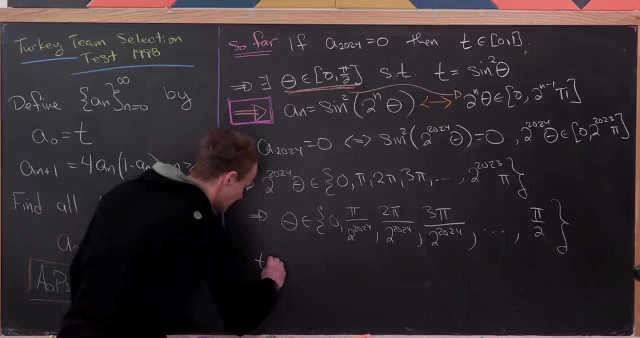 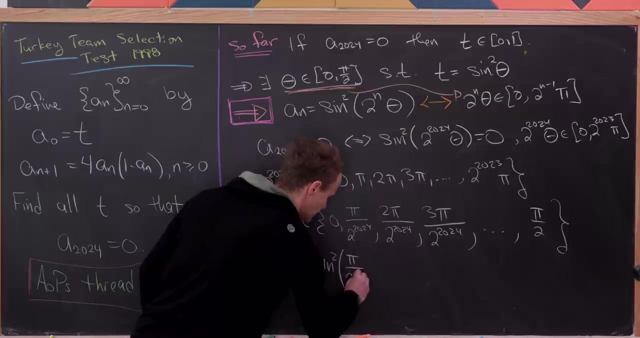 Okay, but we don't want the values of theta, We want the values of t that make this happen. But that simply involves That simply involves evaluating this at sine squared. So that means t comes from the set 0, sine squared of that stuff: pi over 2 to the 2024,. 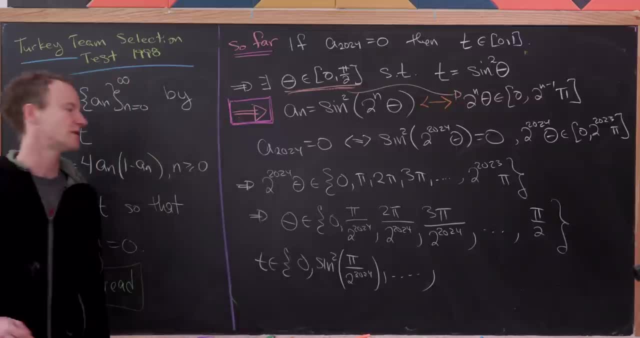 sine squared of 2- pi over 2- to the 2024, so on and so forth, up to sine squared of pi over 2, which is 1.. So there you have it. We have all of the values of t that make the 2024th entry from this sequence. It's equal to 0, and that's a good place to stop.